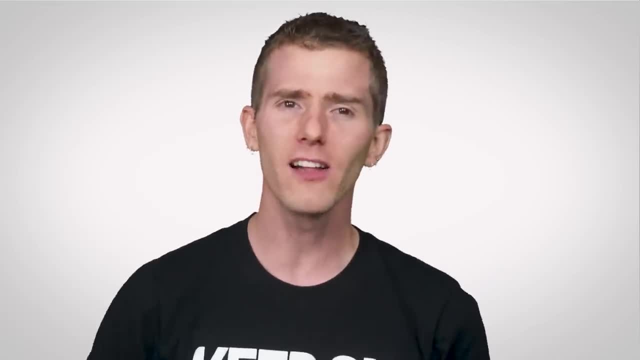 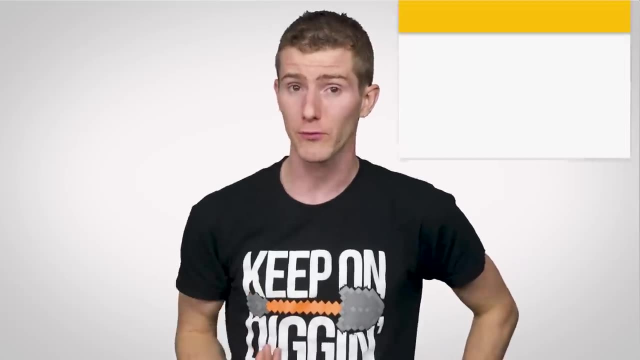 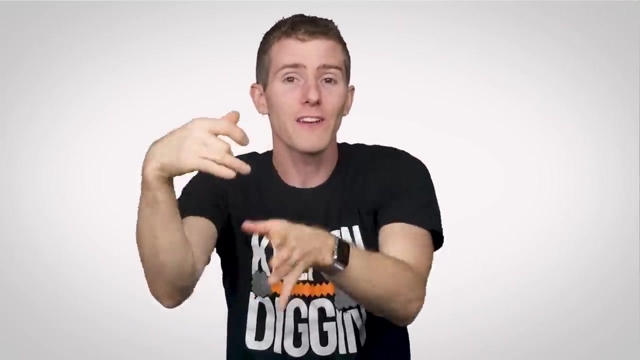 86 megahertz, Kind of like how DSL Internet provides high-speed Internet access over the same wiring as your landline phone by using a different frequency. You can learn more about that up here. And although electrical wiring in your house connects lots of different devices instead of being a strictly point-to-point connection like conventional 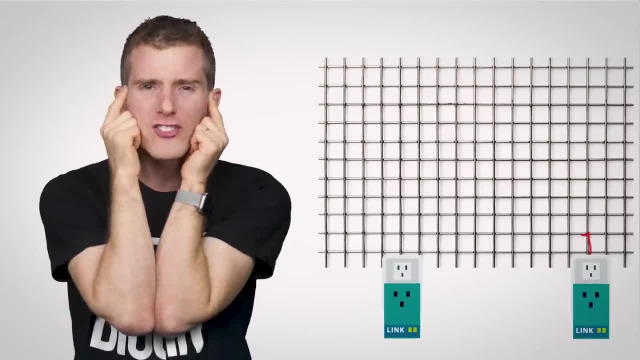 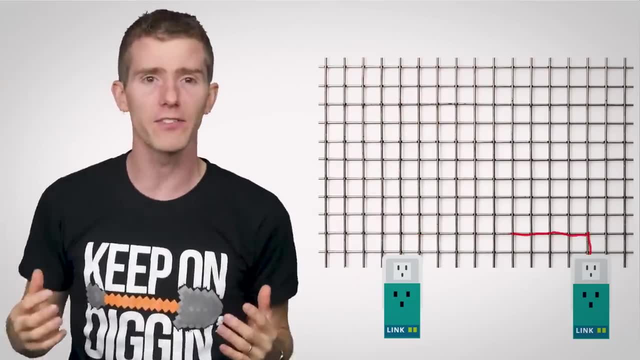 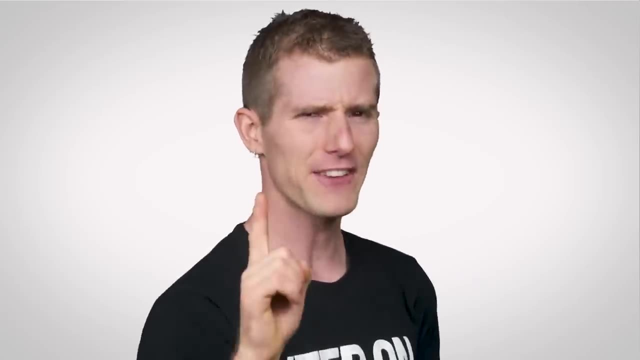 Ethernet power line adapters have internal logic that allows them to catch the signal, Kind of like your smartphone or a laptop can catch a Wi-Fi signal that spreads out in all directions. Well, that's great and convenient and all Linus, but how fast is it? 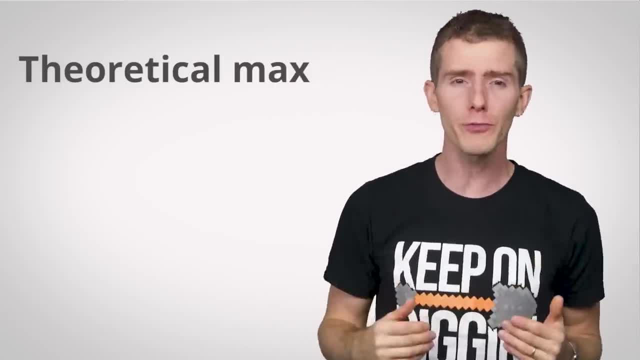 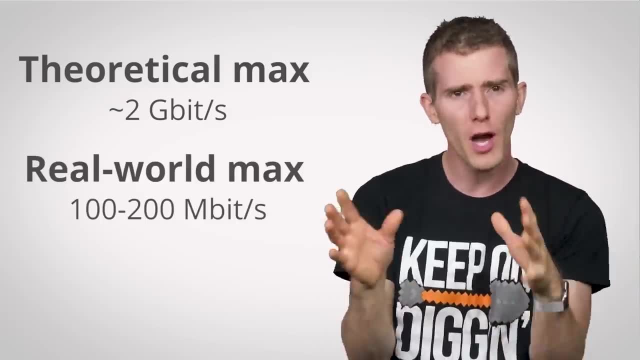 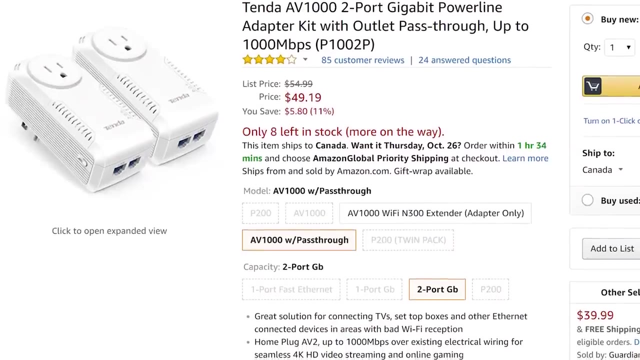 Well, although the theoretical maximum of the newest revision of power line is about 2 gigabits per second, your real-world performance will probably top out at around 100 to 200.. megabits, Although this is still definitely fast enough for high-speed internet browsing and even 4k streaming, and 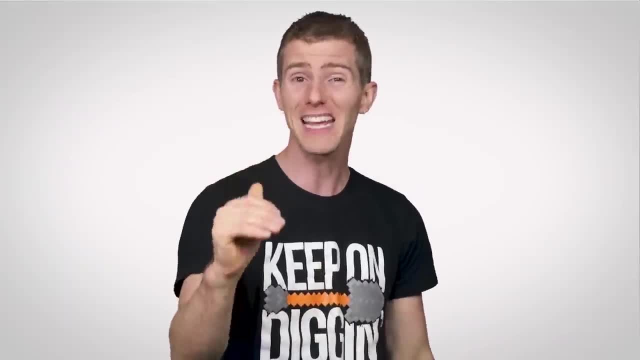 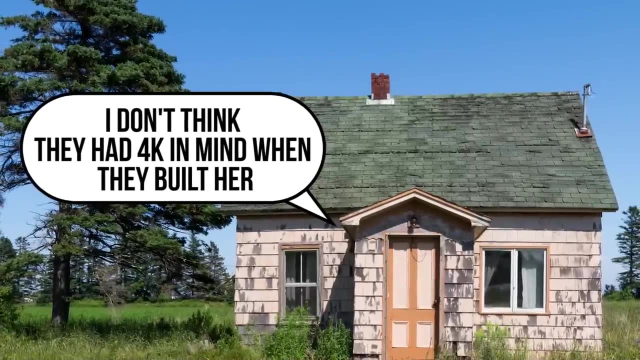 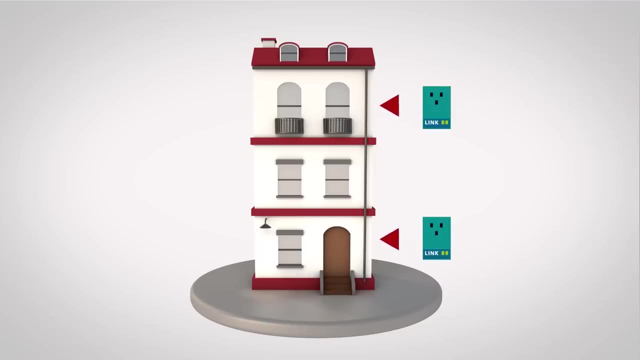 from my personal experience, it comes with a consistency and latency advantage over Wi-Fi. Now, with all that said, if the wiring in your house is older or not the best quality, or if you are trying to place two adapters very far from each other, your speeds might drop well below a hundred megabit. 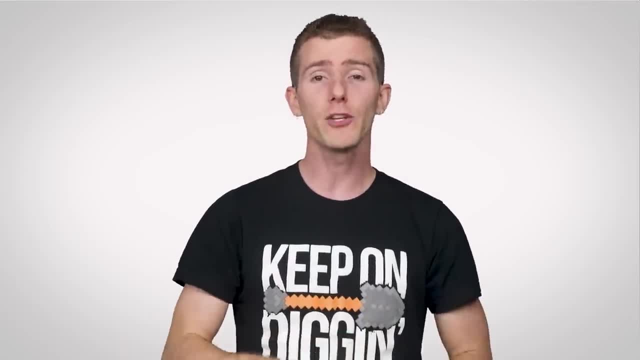 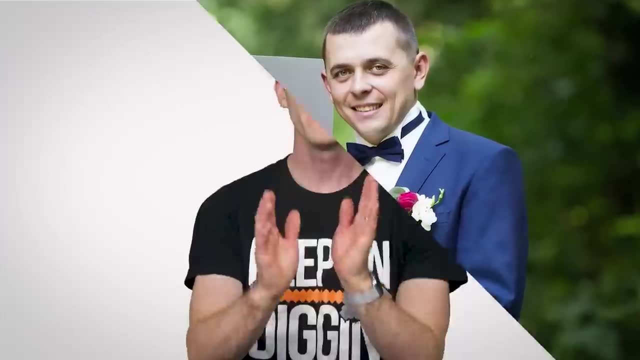 due to signal degradation. So I recommend buying your first couple of power line adapters from a retailer with a solid return policy before making a full commitment. There are also a few caveats to keep in mind when setting up a home power line network. 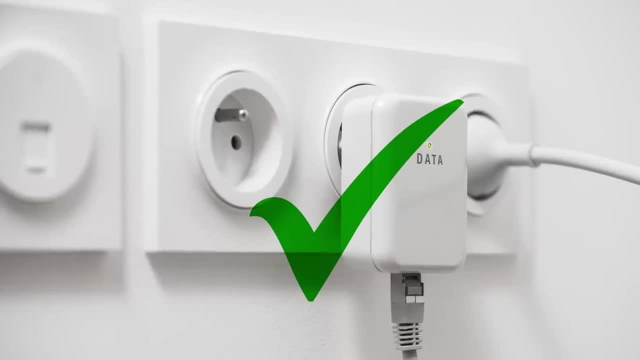 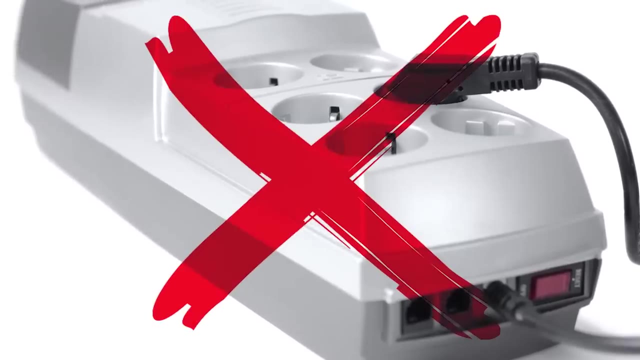 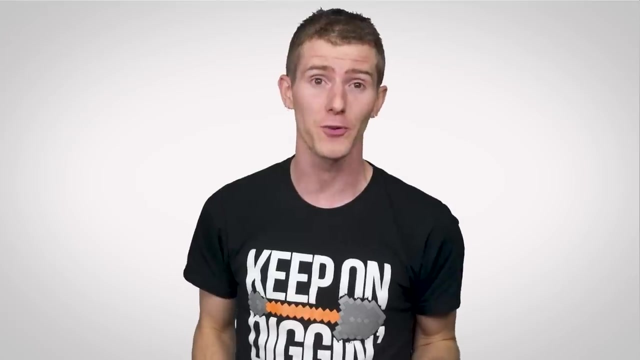 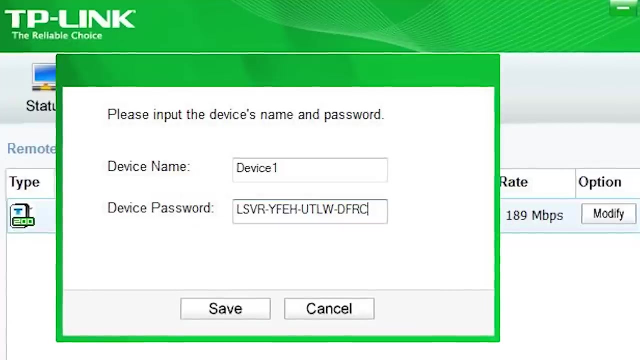 Whatever you do, plug your adapters directly into the wall. Devices like UPS, battery backups, power conditioners and surge protectors can misidentify your data signal as undesirable electrical noise and actually filter it out. Also, be sure to follow the instructions provided for securing your power line network with a password. 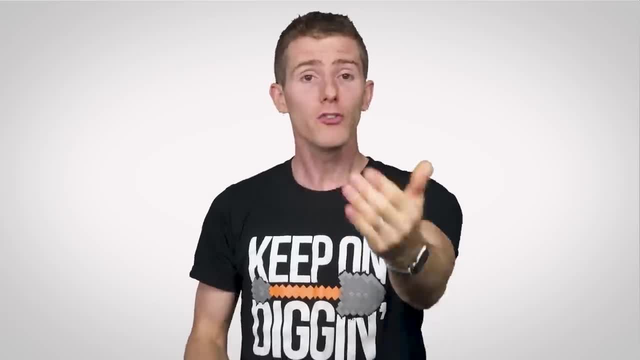 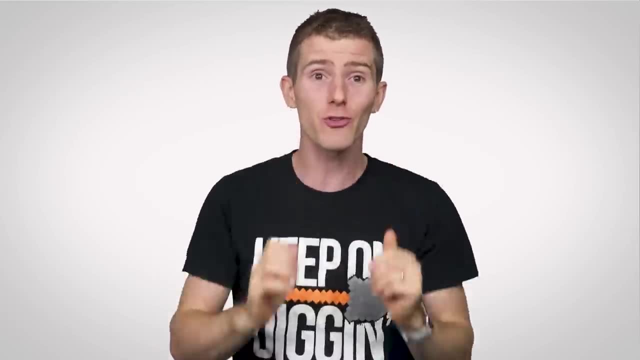 especially if you aren't living in a fully detached home. Just like your neighbor can easily access your Wi-Fi network if it's not password protected. anybody who shares an electrical circuit with you, even through a breaker panel, can possibly get into your power line network.